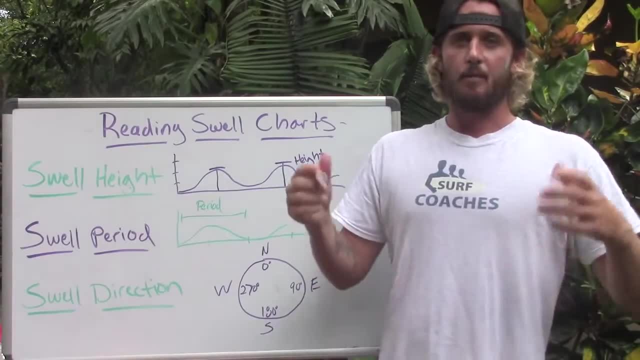 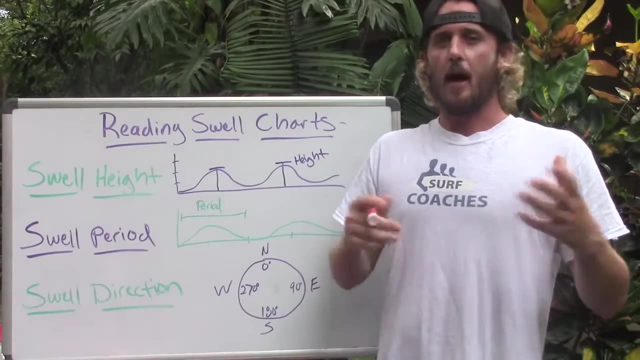 they come from, usually from buoy readings and also from people taking storm models and putting them into the computer and generating these numbers, And I'm going to talk to you about what each one of them means and how they relate to surf in your local area. So the first number you're going to 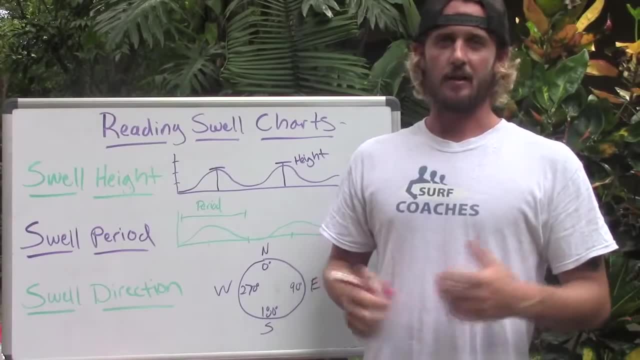 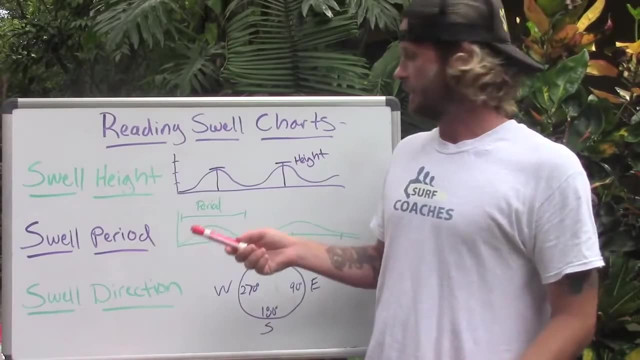 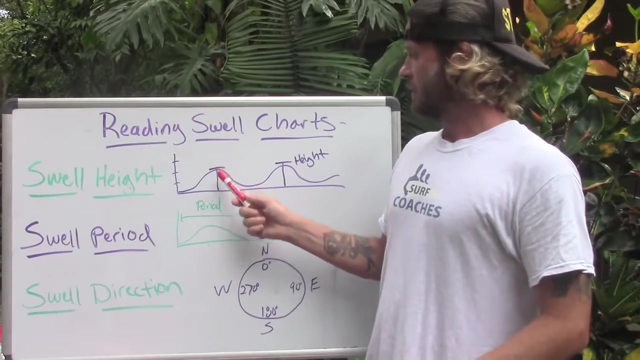 see at every swell forecast is the swell height, And it's usually in either feet or meters. So I have the soil height here and I have a graph here. So the height what that refers to is that's the height measured at a buoy offshore from the base of the wave to the top of the wave. So usually 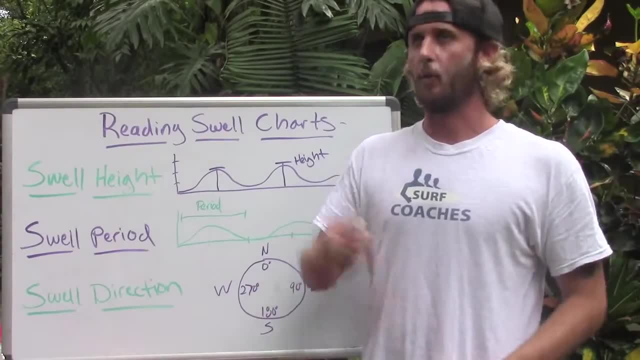 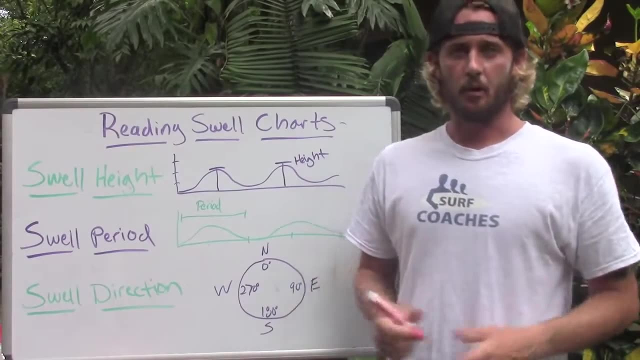 you get in feet or meters, a common reading would be like 2.8 feet, 4.6 feet, And that's the average swell height for waves passing over a buoy. The next number you'll see will be the swell period. So you'll see the height: 4.2 feet, for example, at a certain amount of seconds, And 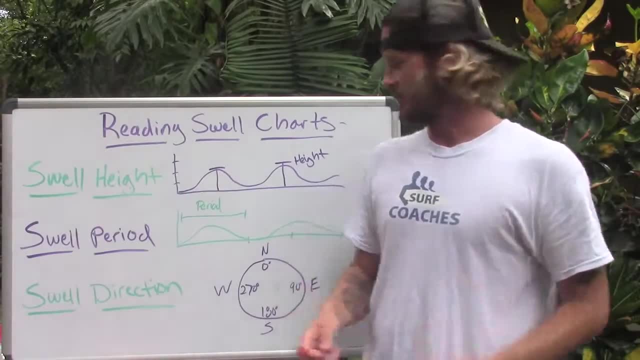 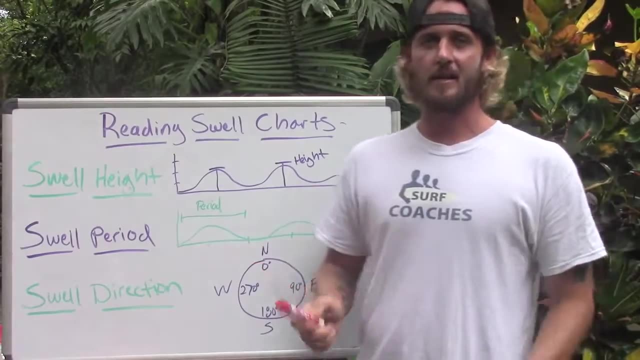 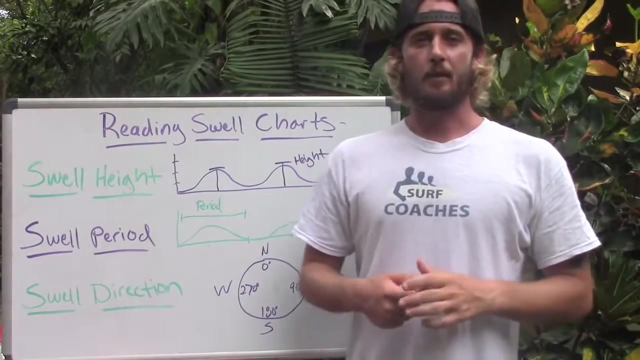 that's a swell period or the frequency. Now, the way they get the frequency is they measure the time lapse between trough to trough or peak to peak. So that's the average amount of time that passes from when a peak of a wave passes a buoy till the next peak, And the last number you'll. 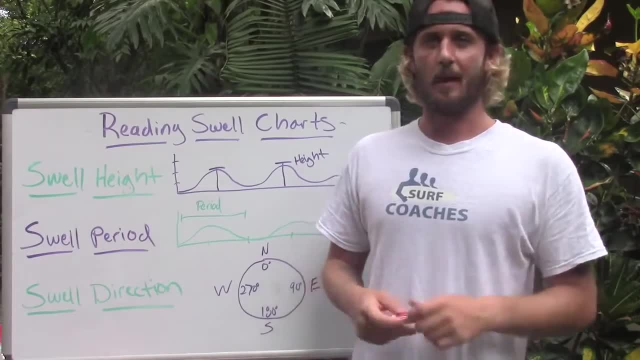 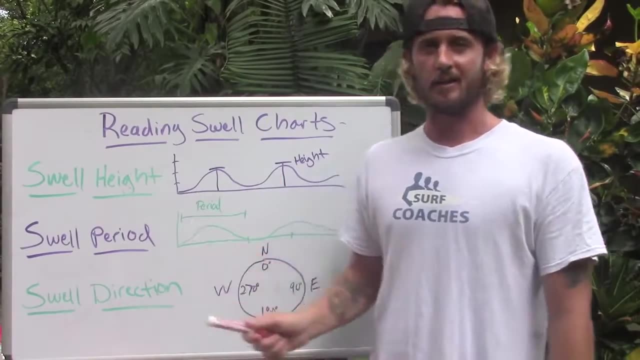 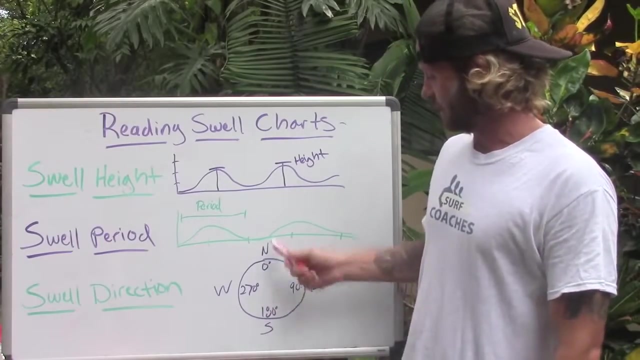 see is the swell direction. It's always measured in degrees, So you might see a surf forecast that says if it's a 1.8 feet at a 16 second period, I'd have 180 degrees. The degrees refers to which direction it is coming from. So I've got a compass kind of thing that drove in here with. 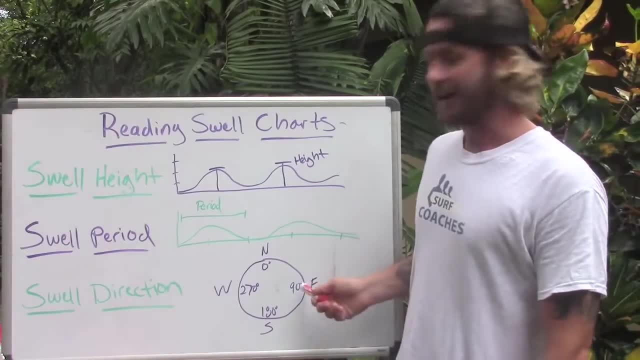 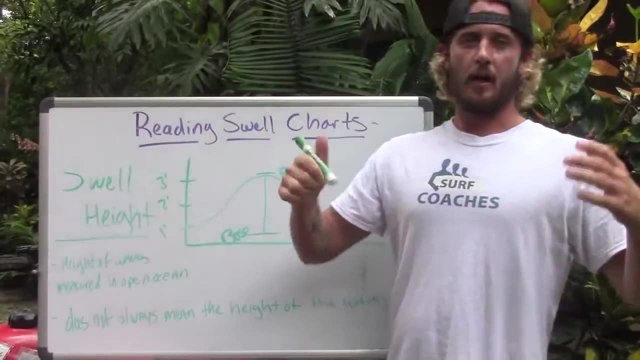 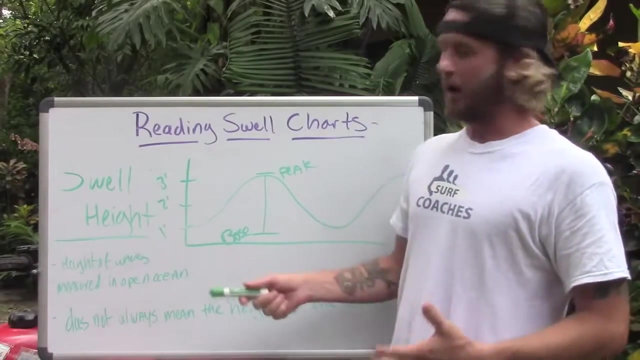 north, south, east, west, and just to note, zero degrees is due north, 90 degrees is due west, 180 degrees is due south and 270 degrees is due west. So the first part of this equation I want to talk about is the swell height. Now, this is most common, you'll see, and this is what a lot of 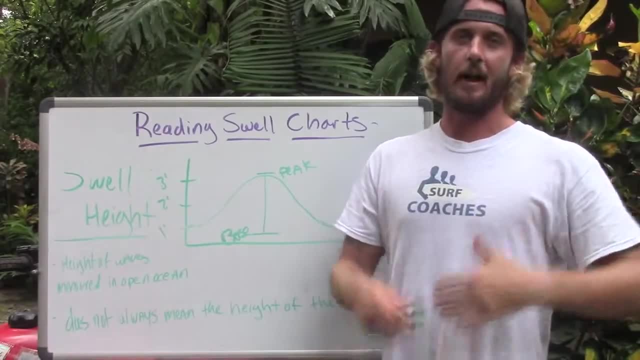 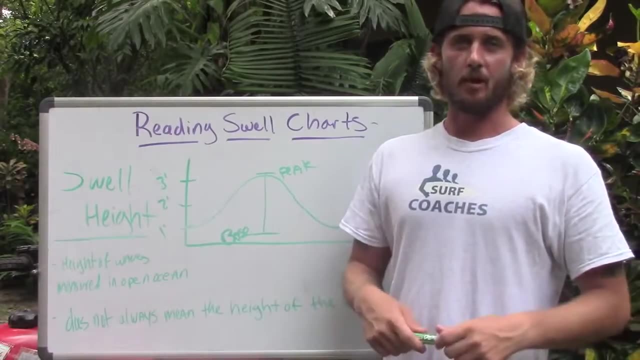 people look at to the height of the waves coming in or the swell coming in out of the open ocean, as measured by buoys or ship readings. Now, the height is usually measured in feet, although sometimes it can be measured in meters, and the height is from the base of the wave to the peak of the wave as it passes. 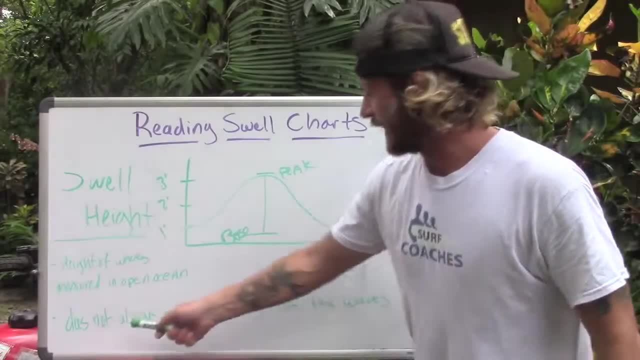 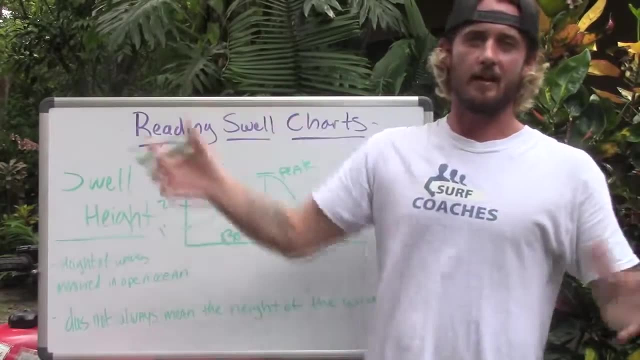 by the buoy. Now, one thing I want to note is that that does not always mean the height of the wave. so you can see a swell reading that says the waves are 10 feet at whatever seconds, and sometimes people say, oh, the waves are going to be 10 feet tomorrow. That is not always true At the same. 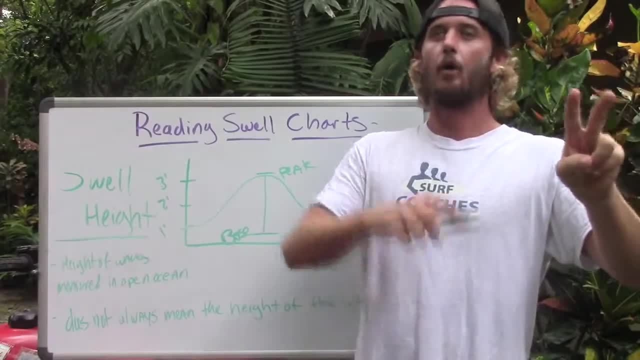 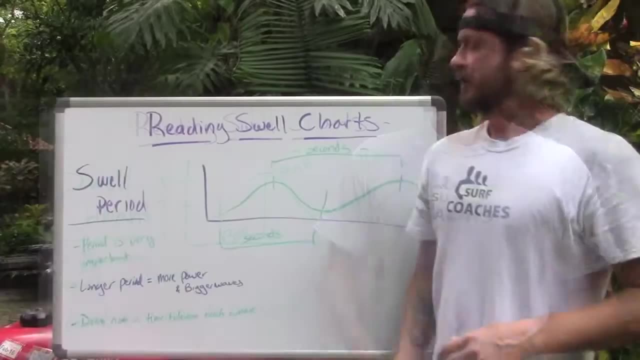 time the waves can say that it's going to be a two feet at a longer period, and that doesn't always mean that the waves are going to be two feet, because it's really dependent on the period which we're going to talk about next. So the next part I want to talk about is a swell period and in my 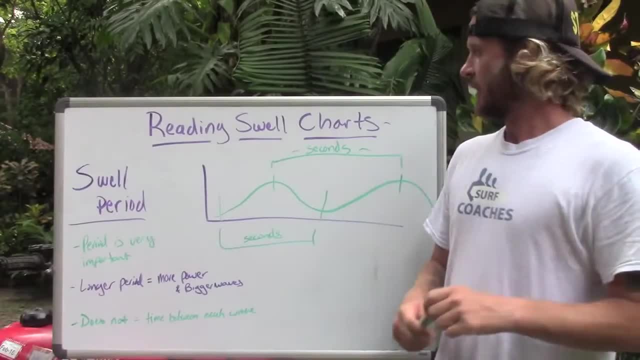 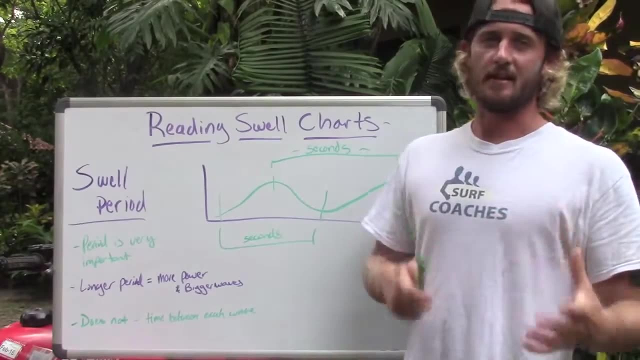 mind the swell period is one of the most important things about reading a swell forecast. So just to get for starters, when you look at a swell period, swell period is measured by the buoys offshore and that measures the distance in seconds from trough to trough. so the low points of each wave. 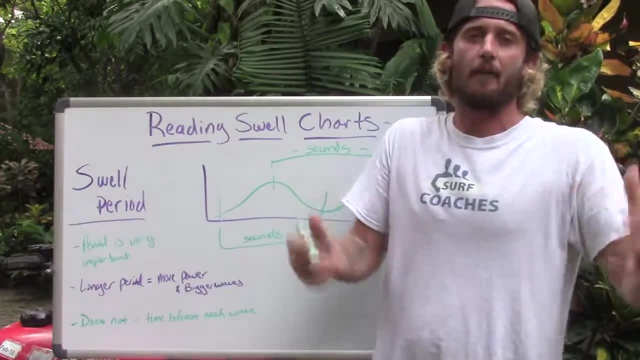 or from peak to peak. It really measures the distance from trough to trough and that measures the distance from peak to peak. It really measures the distance from peak to peak. It really makes no difference and it basically takes an average over time. So the period is probably one of the most 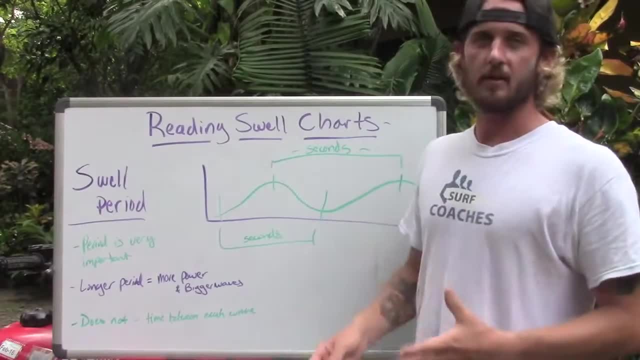 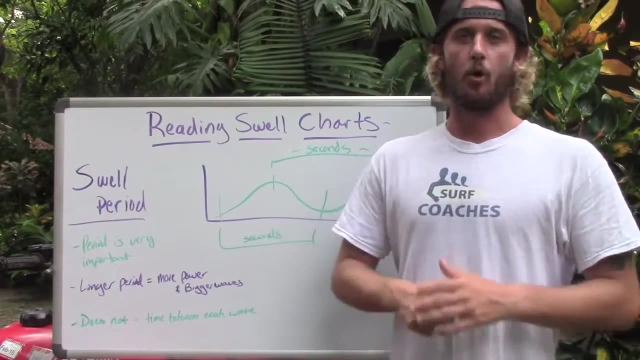 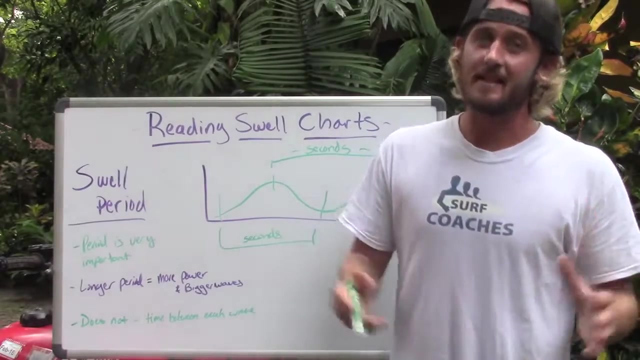 important parts of the swell, because the period directly correlates to how much energy is in the swell. So the longer the period, the more power in the bigger wave. So a swell, for example, that has two feet at eight seconds and a swell that has two feet at 16 seconds is going to have way more than. 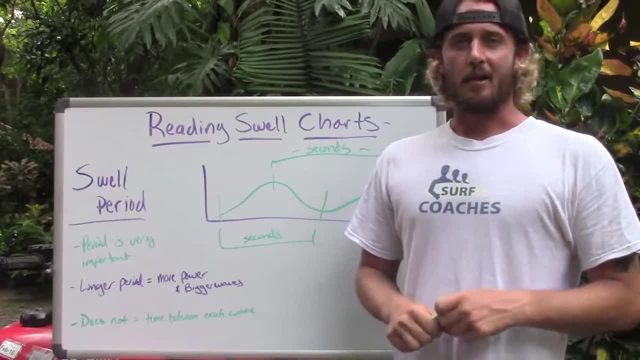 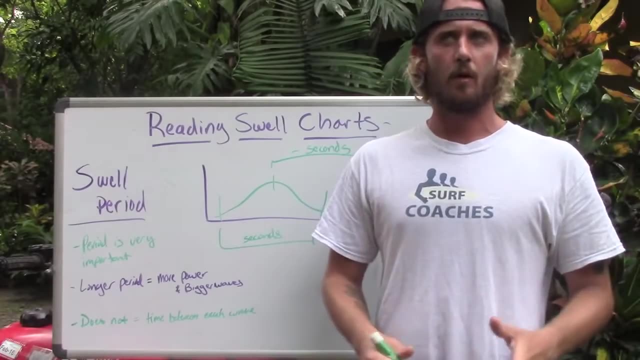 double the power in each wave. One other note I want to make about the period. that's a common misconception. people ask all the time. I say, okay, tomorrow the waves are going to be only two feet at 14 seconds. They say, well, I went out surfing but the waves weren't 14 seconds apart. Well, that's not. 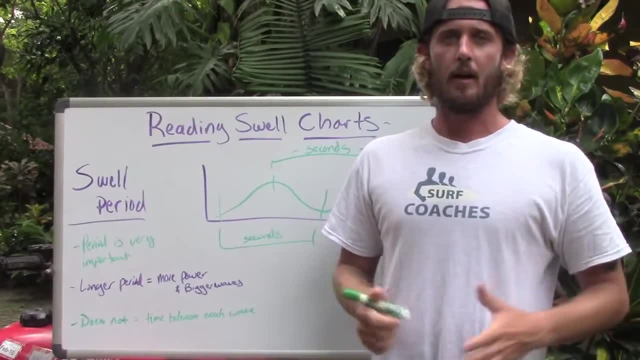 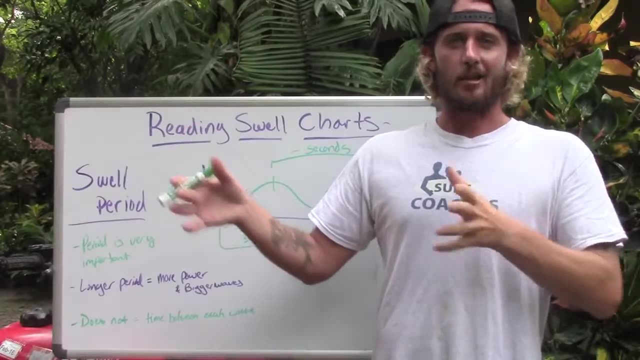 exactly what that means. Again, these are readings that come from buoys that are offshore and it measures the mean distance, the average distance between peak to peak, trough to trough, and as the wave approaches the beach it actually kind of changes and I'm going to show you guys that in 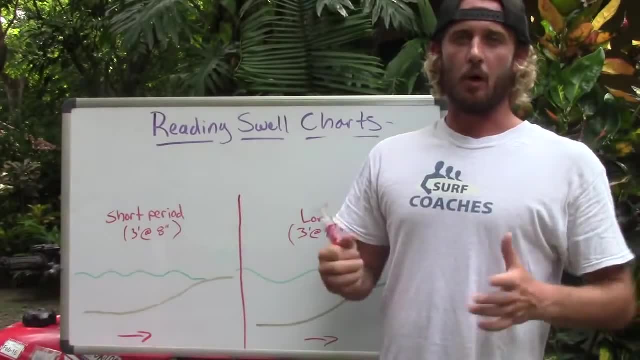 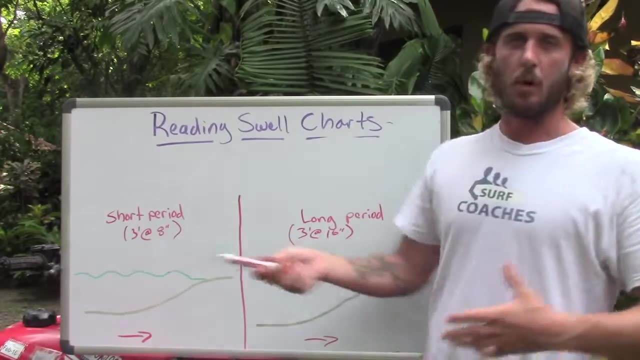 the next segment. So now what I want to talk about is swell period and why the period of the swell is different to forecasting waves. So what I have here is a short period swell and a long period swell coming on the same beach- a nice sloping beach break- and the waves are both coming in this. 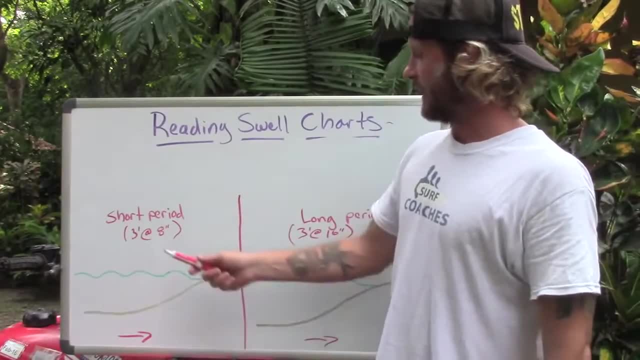 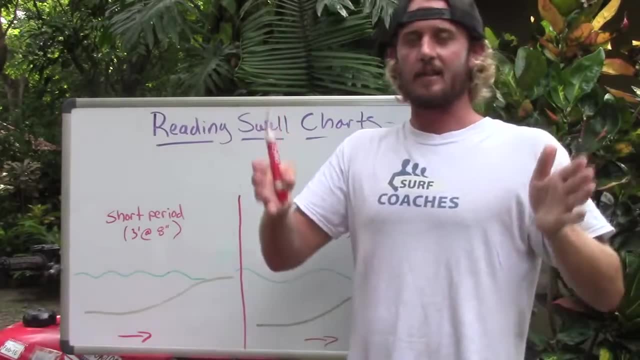 direction. So we'll start with a short period swell. So these swells are the same height, three feet. this one's three feet at eight seconds. so that means that the height of the swell at its peak out in the open ocean is three feet and the distance between waves as the swell train moves in. 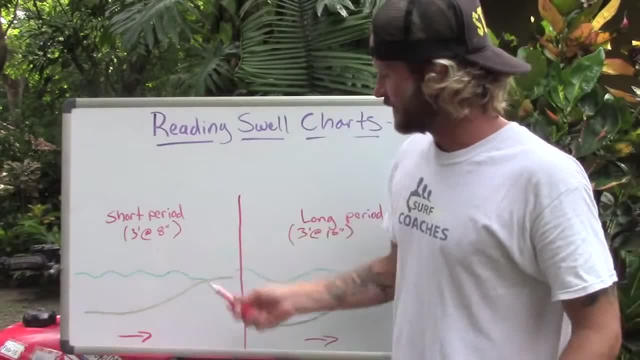 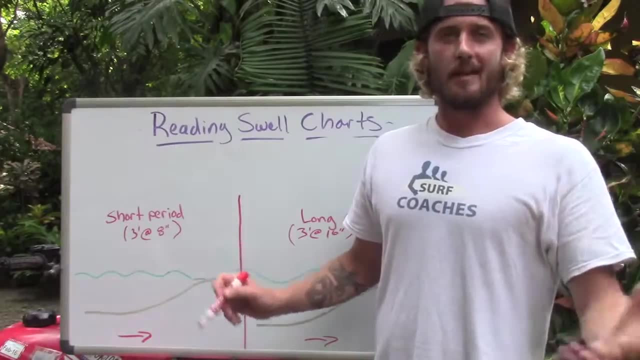 is eight seconds between peak to peak. So as this wave moves in, what happens is this front part of the wave starts hitting the beach kind of early. it starts slowing down and encounters friction. So as this front part of the wave hits the beach, it starts slowing down. but the back part of the wave 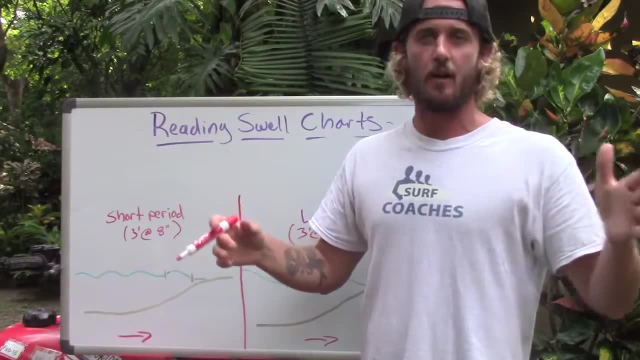 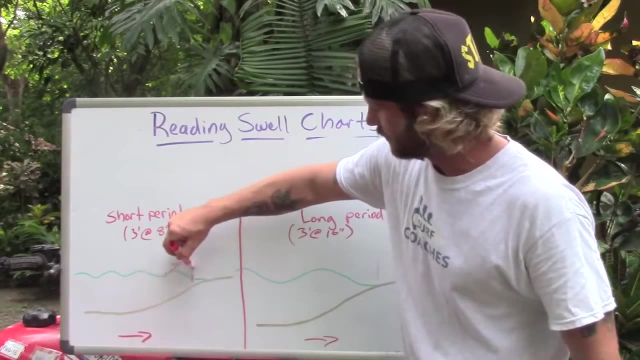 back here eight seconds later is still moving much faster because it hasn't encountered the same friction. So what it does is it builds up as it moves here, so it causes the way to build up into a breaking wave and on average, a wave that's three feet at eight seconds will turn. 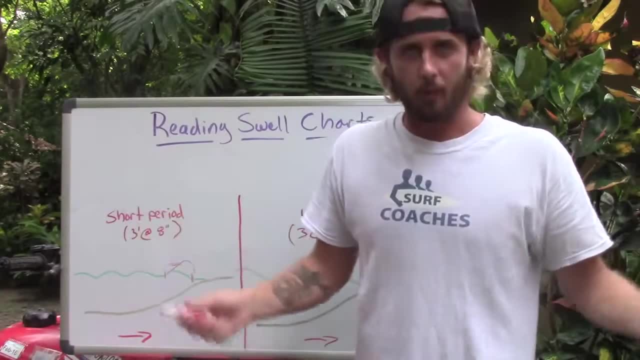 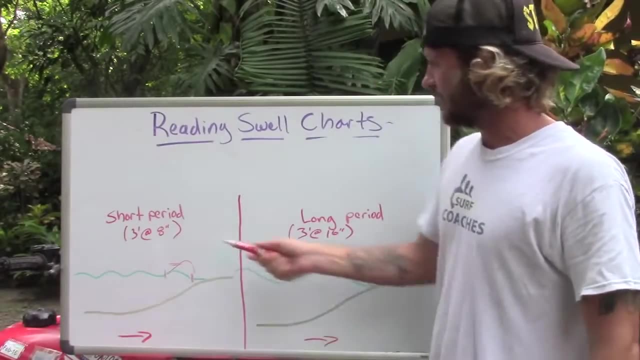 into about a two to three foot wave on your average beach break. Now, when we look at a long period swell, the same swell height out in the open ocean- three feet, okay, from base to the peak, but now the swell period is 16 seconds, so it's double the distance. 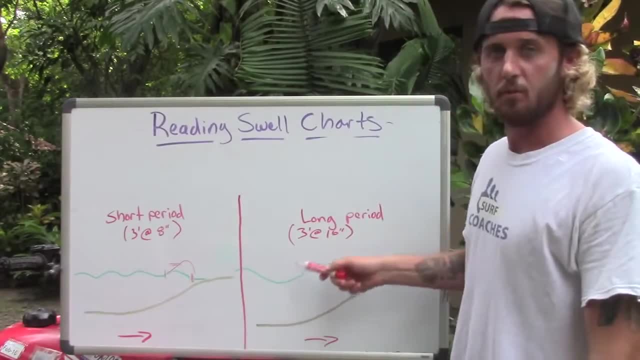 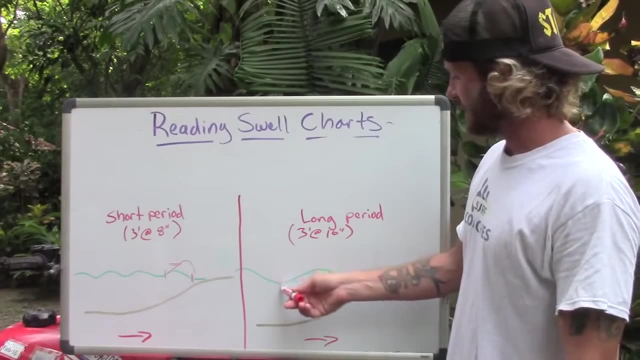 So why is that important? Well, as this wave moves, moves towards the shore, the front part of the wave starts slowing down, just like this one, and then the back part of the wave is 16 seconds behind it, and it's so much longer of a wave that the wave builds up more and more, so the it's almost like a 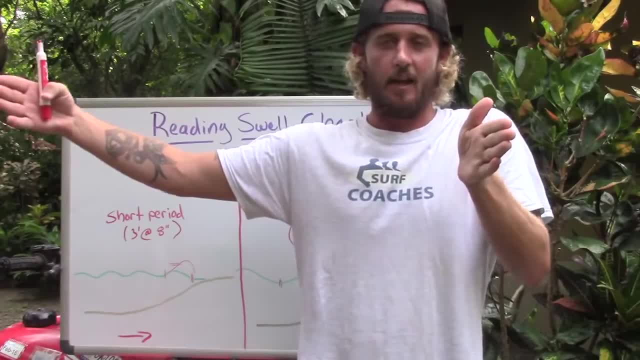 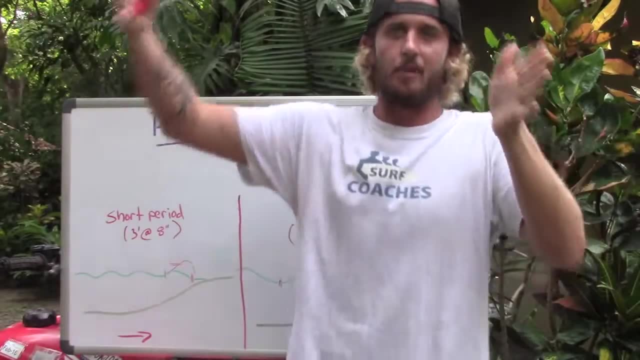 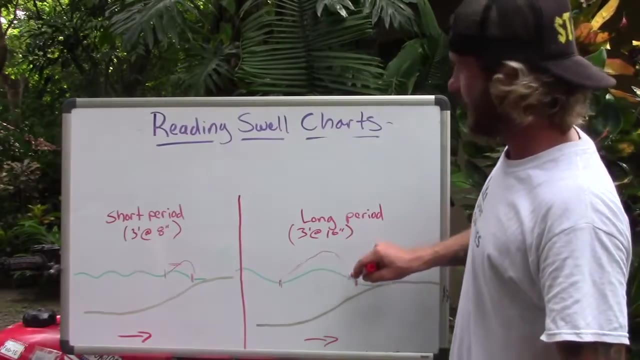 train wreck or a car wreck on interstate, the first car wrecks and if you only have five cars and they pile up, versus if you have 15 cars and they pile up, it's going to be a bigger build up. so basically all what's happening is this is building up even more because this part is moving so much faster and a 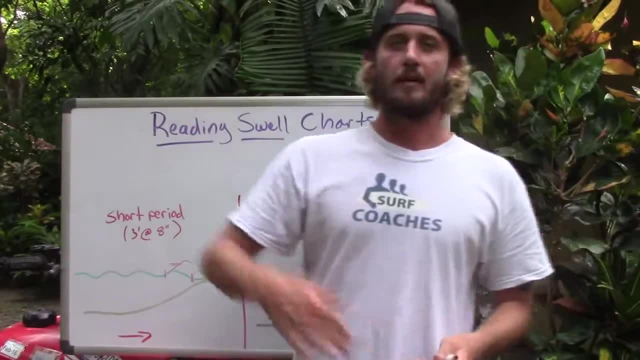 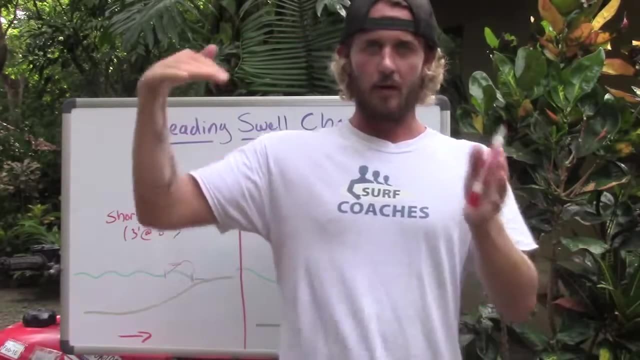 good analogy can you can think of is if you were riding down a hill on a bicycle. so you're riding down a very mellow hill and you're going down the hill and you run into a brick wall. if you're going really slow, you're only going to get tossed out a little bit, whereas if you're going down a steep hill, 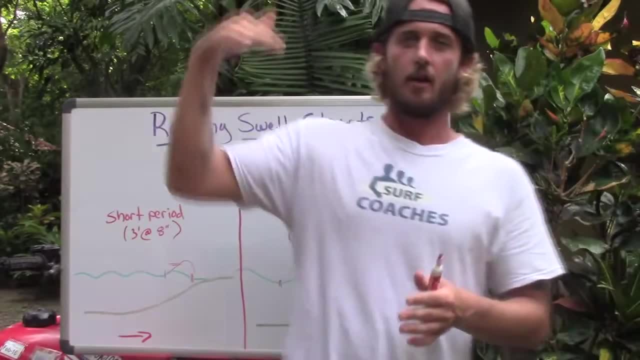 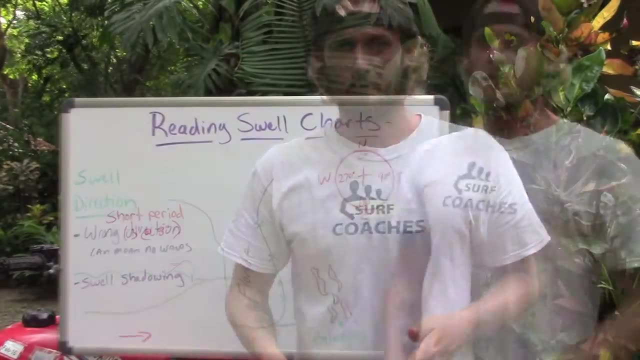 and you're moving much faster. which long period swells move, faster you're coming down. you're going to hit the brick wall stop, just like the front of the wave stops, and the back's going to fly up even more. so the last thing I want to talk about today is swell direction and explain why swell. 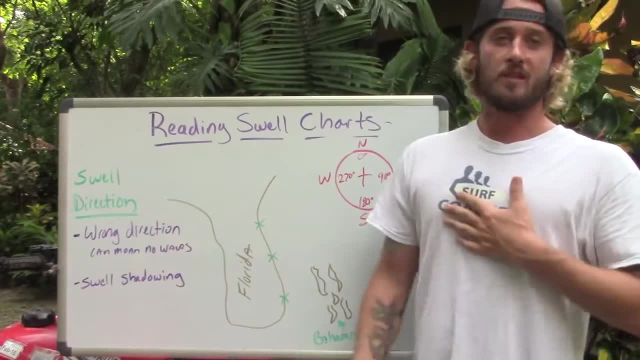 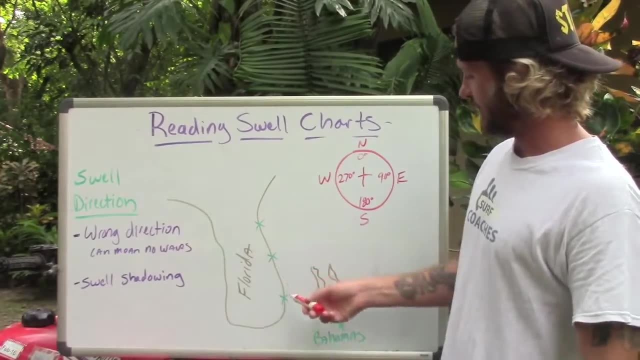 direction is important. so what I did is I drew a diagram of my home state of Florida and I'm going to explain how swell directions affect ways to come in here. so I drew a couple places. you have North Florida, Central Florida, South Florida. If you look at the state here, we also have the Bahamas offshore and I'm going to explain why. 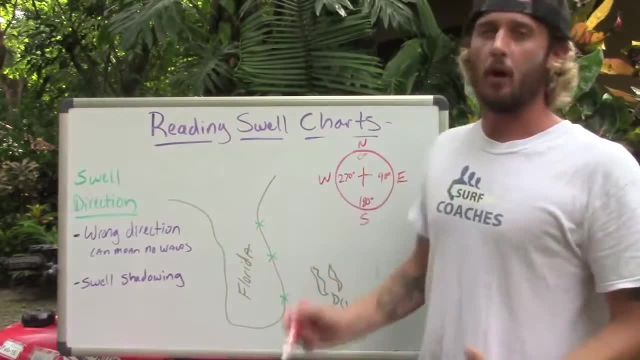 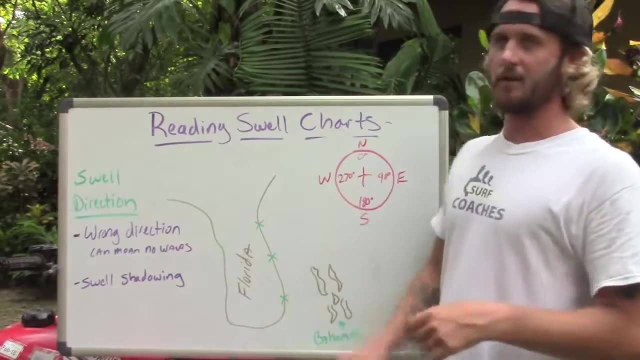 swell. direction is important because if you have the wrong direction it means you can be completely blocked from swell or the swell can't make it into a certain area. so what you'll see is when you look at a swell it'll say maybe three feet at 16 seconds, and it'll give you degrees. so the 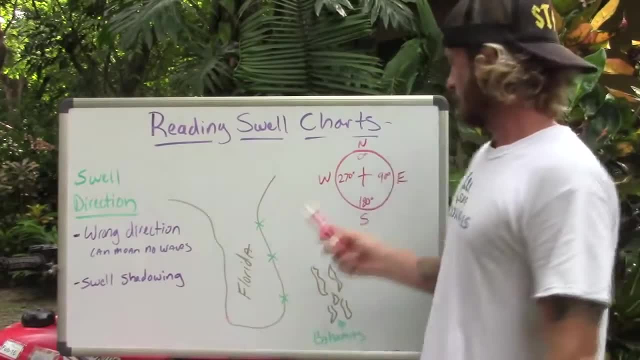 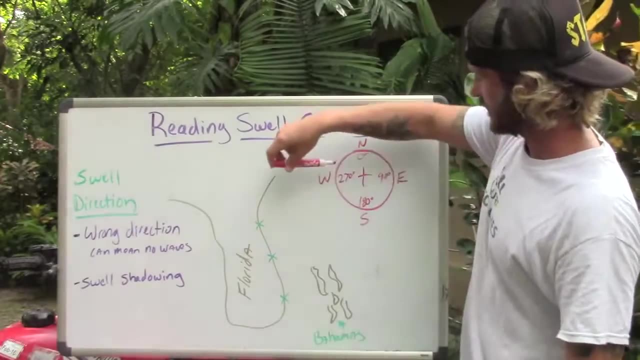 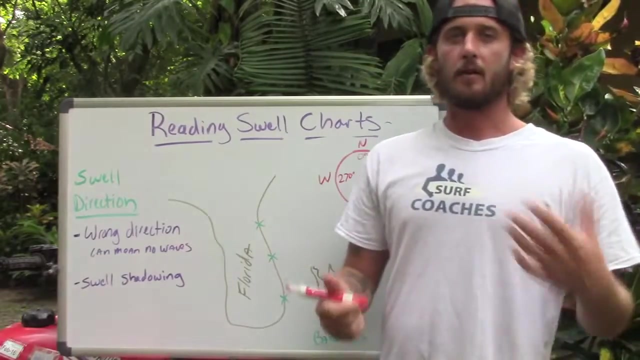 degrees will be, say, 90 degrees. so you can look at this and know that 90 degrees swell, a swell out of the west. if the swell is coming straight from the west it'd be 270. coming straight north, zero degrees South, 180.. so why is that important? well, over the years I've had friends come to me and say: Brent, the 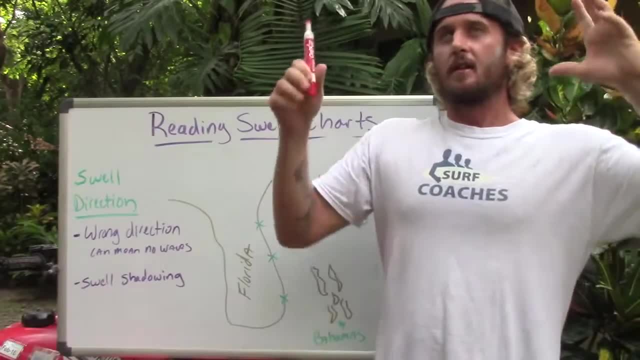 waves are going to be so good. tomorrow it says it's going to be 10 feet at 12 seconds, and there's the ways you're going to be great. and I go to look at a swell forecast and they're right: it's 10 feet. 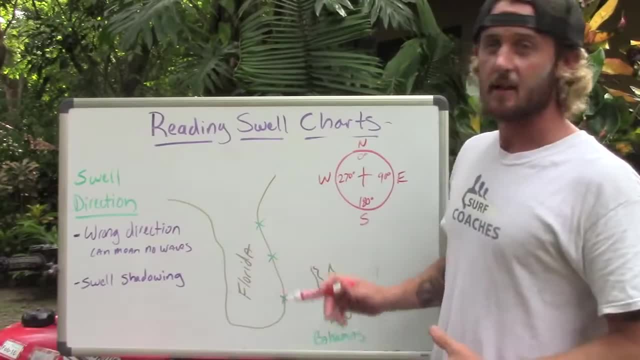 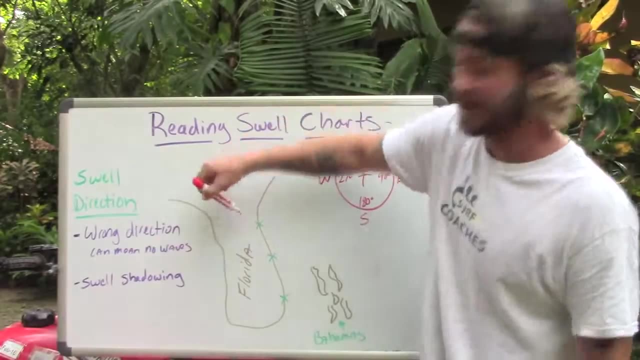 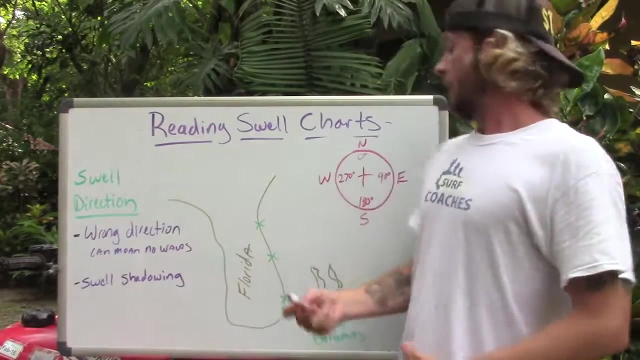 at 12 seconds, but the degrees is 270, which means the swell is out of the west. so if I'm here here and the swell is coming from this direction, guess what? there's no real swell. that means the wind and the swell is all blowing out to sea, which means no waves at your local break. so if that same swell 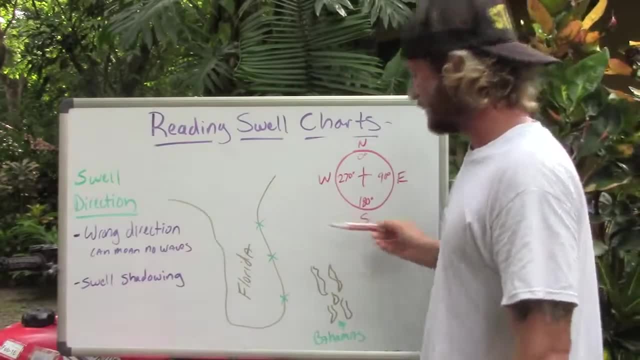 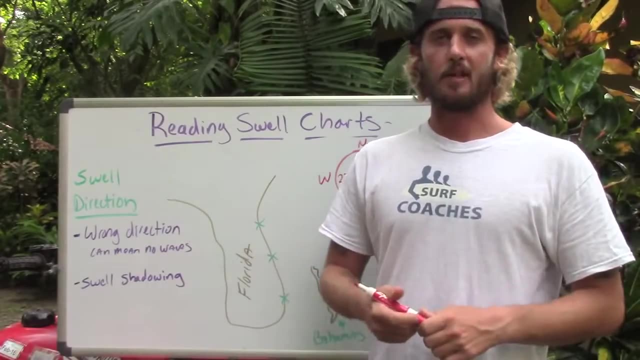 were to turn around and be out of 90 degrees out of the east, that means swell is going to be coming straight out of the place at any of these directions. another reason swell is important is our soil direction is important is because we often have islands offshore that can Shadow or 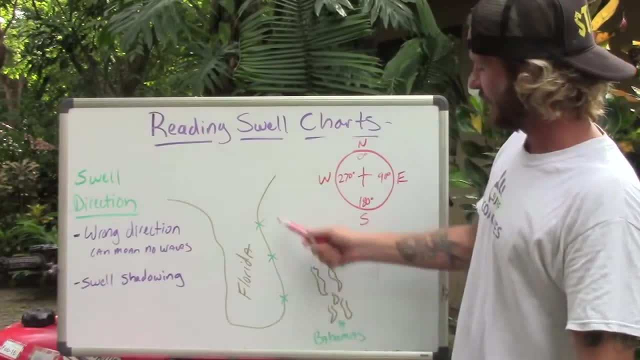 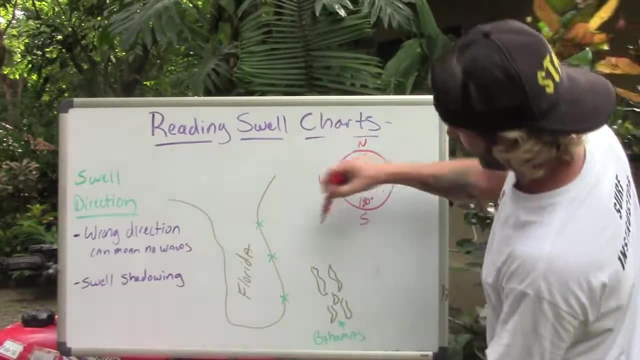 block swell. so we'll look at this diagram again. we have three different places in Florida. so say the swell is coming out of 90 degrees out of the due East, coming straight at Florida. well, guess what? if you're here in Central Florida or North Florida, the swell is going to be able to come in without. 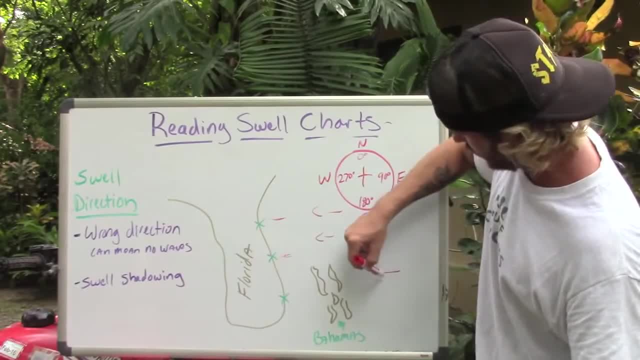 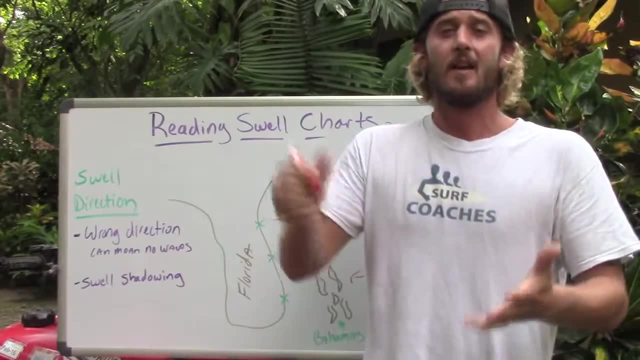 getting blocked at all, whereas if you're here in South Florida, guess what the swell is coming in and then it gets blocked by the islands offshore. now this is very common in places in England, in Southern California and, of course, here in Florida. so knowing the swell direction is very important.